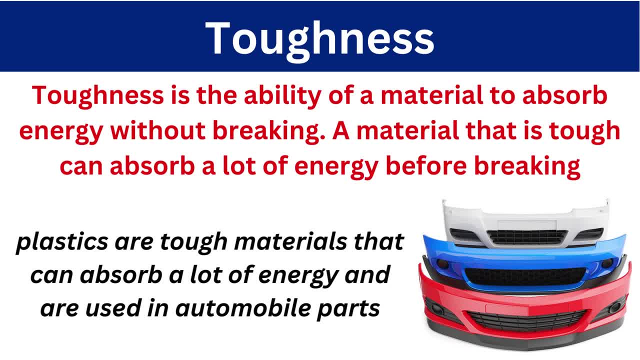 that can absorb the lot of energy before the breaking. Okay, and you can take the example: plastics are tough material that can absorb the lot of energy and are used in the automotive part. Okay, if you see, now, nowadays the car bumper is made up of the plastic material, because that material can absorb the maximum. 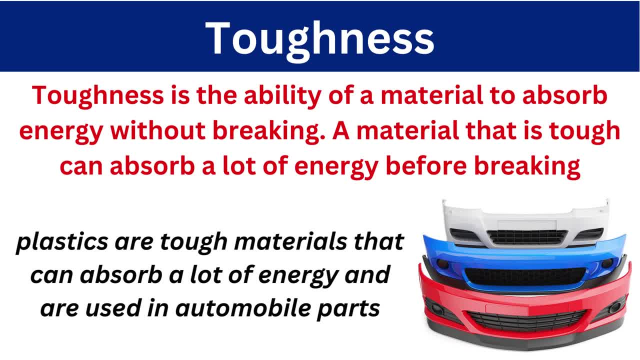 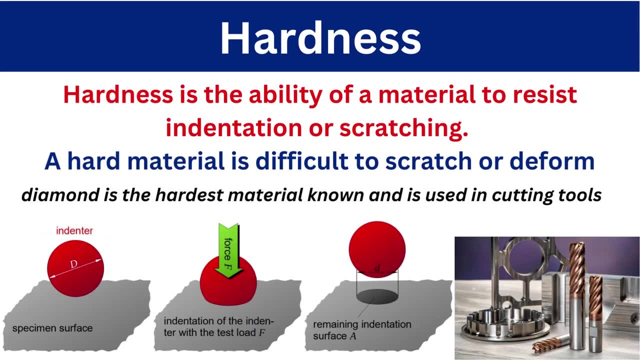 energy, maximum energy, during the impact loading. So whenever our component under the impact loading, at that time toughness is very important. properties, Okay. property of material, Okay. Next one, we have hardness. So hardness is the ability of material to resist energy without 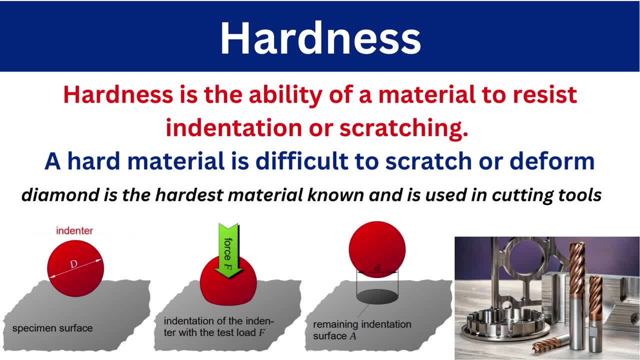 indentation or scratching. Okay, so hardness is nothing but the ability of material. it raises the resist, the scratching. Okay, so the hard material is difficult to scratch or deform. Okay, If you take the example of the diamond: Okay, so the diamond is the hardest material and it is used in the cutting tool. 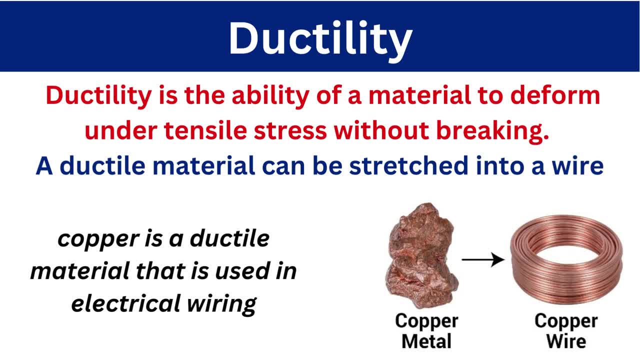 ductility. So the ductility is nothing but the ability material to deform under tensile stress without breaking. okay, so without breaking it will deform. okay, under the tensile state it will deform, but it will not break. okay, so ductile material can be stretched into a wire, okay, and you can take example here: copper is the ductile material that. 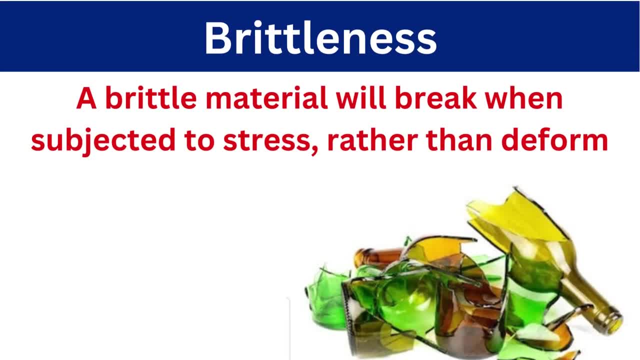 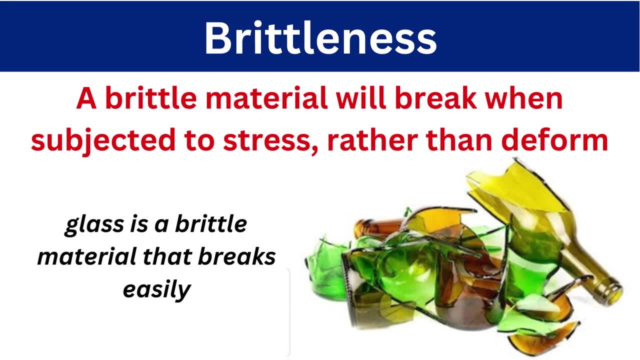 is used in the electrical wire. so next one is a brittleness. so brittleness is the opposite of ductility. so the brittleness material will break when subjected to the stress. okay, ductile material, uh, when it is subjected to tensile load, it will, uh, it will deform, but uh, it will not break. okay, but. 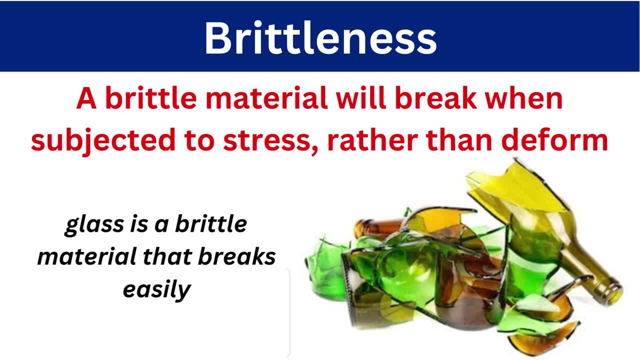 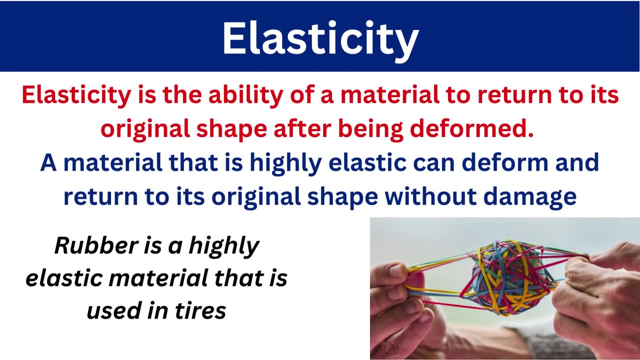 in a brittle brittleness. the brittle material will break when subjected to the stress. uh, so it will not deform? okay, directly, it will. suddenly it will break. you can take the example of glass. okay, glass is a brutal material that break easily. okay. next one is the elasticity. so the elasticity is the ability of material to return to its original. 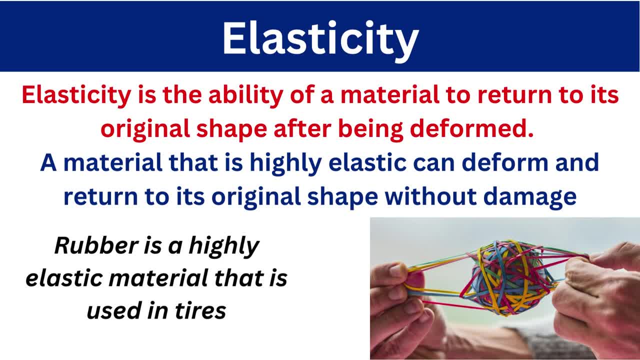 shape after being deformed? okay. when we are subjected to the load, it will deform. okay, and once you release the force, it will regain its original shape. okay, so the material that is highly elastic can deform and return to its original shape without damage. okay, so rubber is the best example for 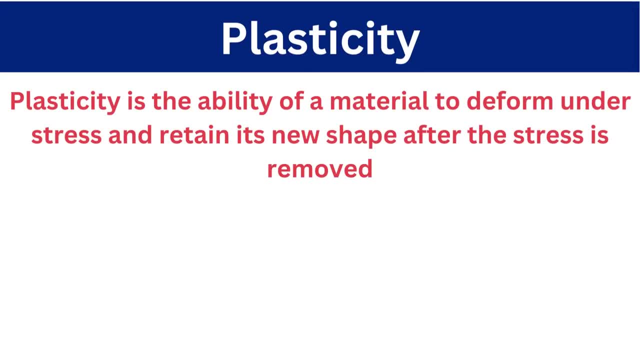 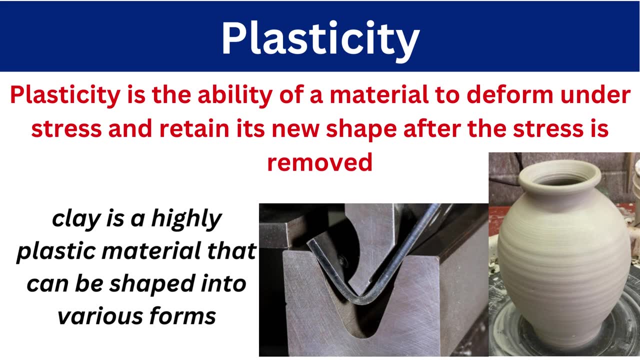 right me also. this is one or both the products that can eliminate the resistance. also, if you really use this side, Donkey can adapt this side which is got to there, this side here as well. okay, so that is easier at the beginning rate, which is excessive force it is therefore 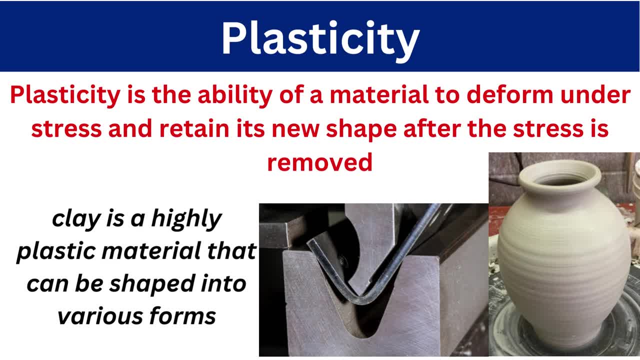 very efficient. but, uh, this is another uh technique that you might find, basically theνbени. okay, that, so that is our application. okay, now let me explain the biggest mistake: that we read the shape. okay, so you can take the example of clay. okay, clay is a highly plastic material that can. 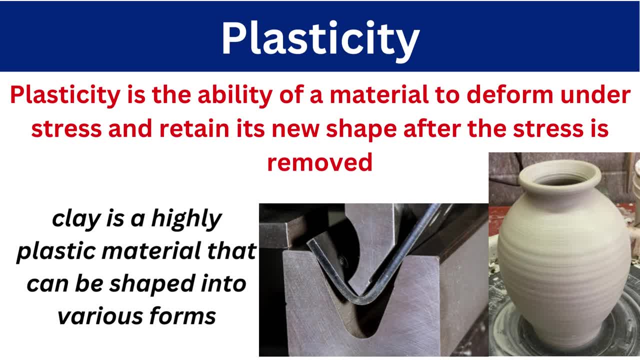 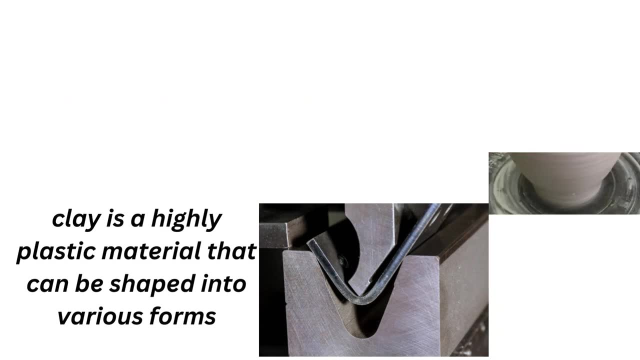 be shaped into various form. so the plastic plasticity is very important for the sheet metal component. so whenever we are, we are applying the force so that, because of the plasticity, it will not regain its original shape. okay, so next one, we have the fatigue. so fatigue is the ability. 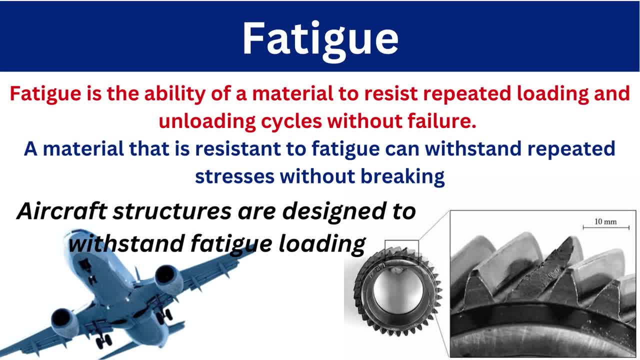 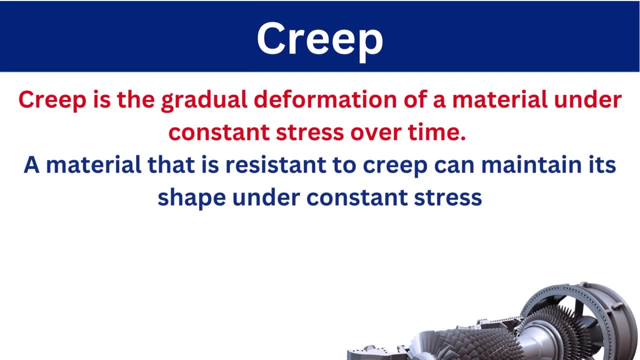 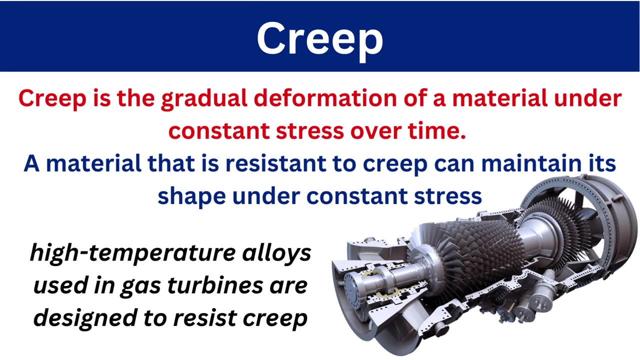 of material to resist the repeated loading and unloading cycle without failure? okay, so the material resistance to the fatigue can withstand the repetitive stresses without breaking aircraft structure are designed to withstand the fatigue loading, okay. next very important property is creep. okay, creep is the gradual deformation of material under the constant stress over a time. 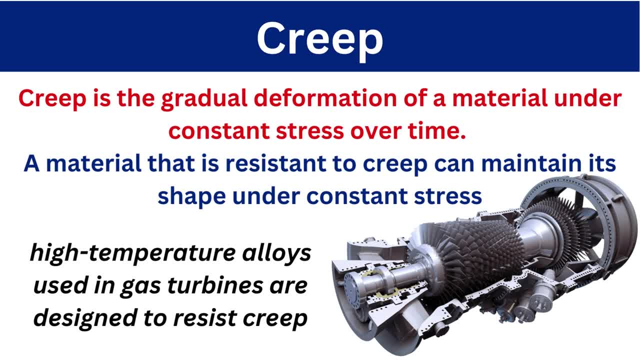 okay, so the material that is a resistance to creep maintain its shape under the constant stress? okay, and you can take the example of a high temperature alloy using the gas turbines are designed to resist the creep, because the creep is a gradual deformation of material under the constant stress over the time. so suddenly,